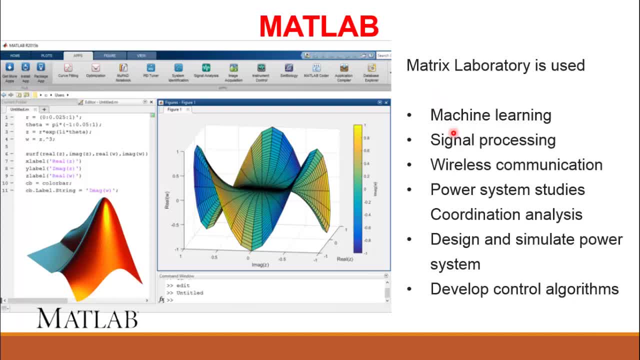 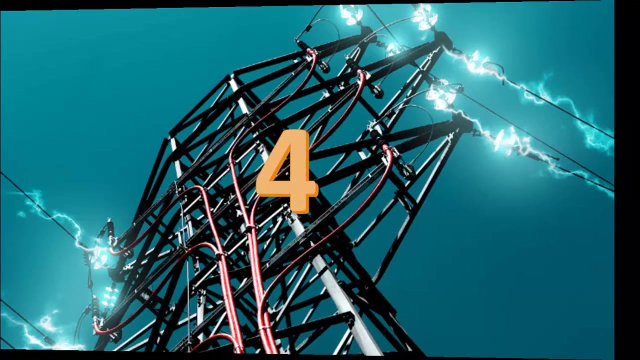 of the electrical engineering, Which involves machine learning, signal processing, wireless communication, and, above all, it also covers the power system studies, coordination, analysis. You can also design and simulate power system and also develop control algorithm for the power systems. Next on our list is the Simulink. The Simulink is a sub part of a MATLAB and it is basically. 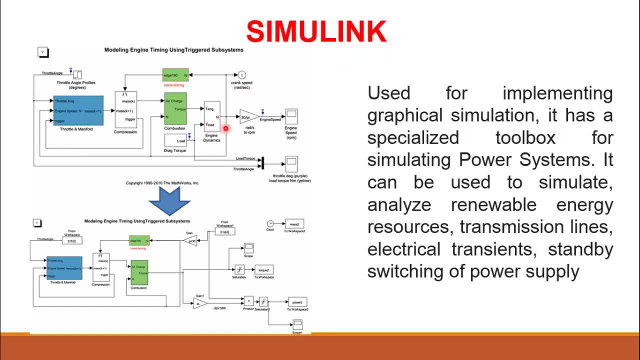 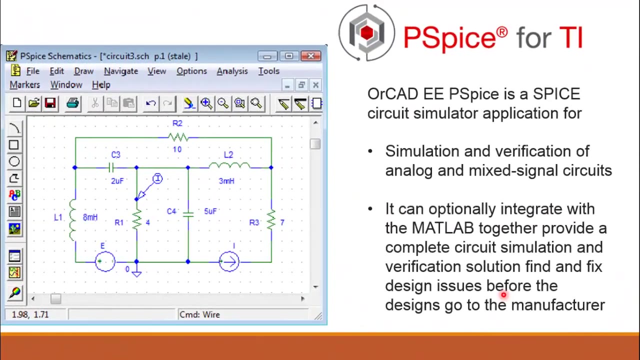 a block representation software. This software is used for implementing graphical simulation. It can be used to simulate, analyze renewable energy resources, transmission line models, electrical transients and standby switching of power system. The next is the PSPICE or the ORCAD WP-SPICE is a circuit simulation. This is a circuit. 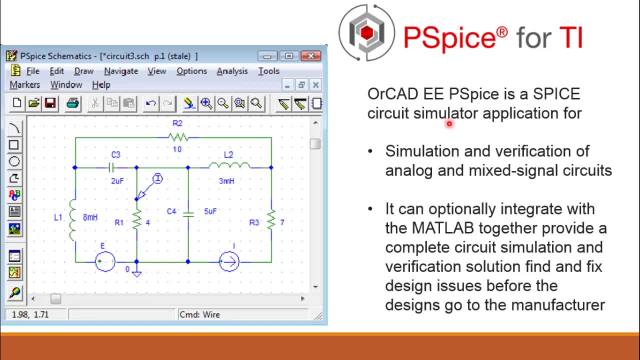 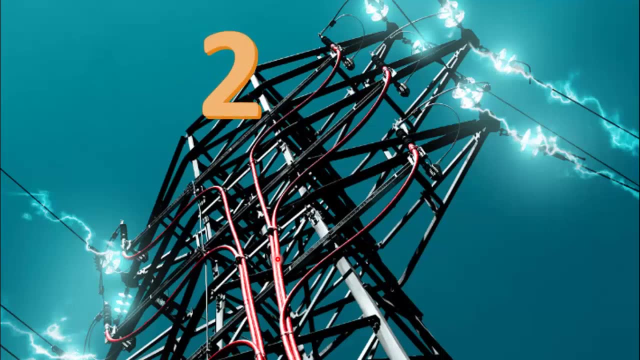 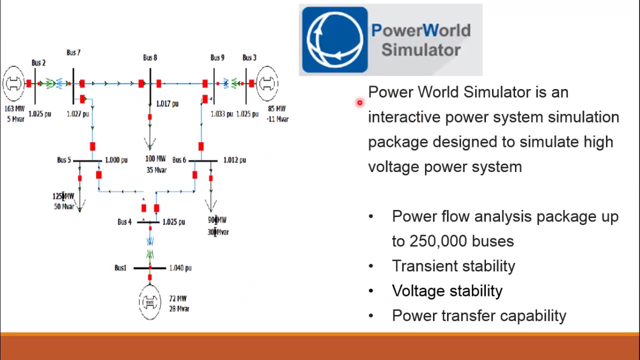 simulation. This is a basic application for the electrical and the electronics engineer. Here you can draw a basic analog circuit and after that you can perform simulation and verification of analog and mixed signal circuits. The second on our list is the Power World Simulator, and this is a very important and 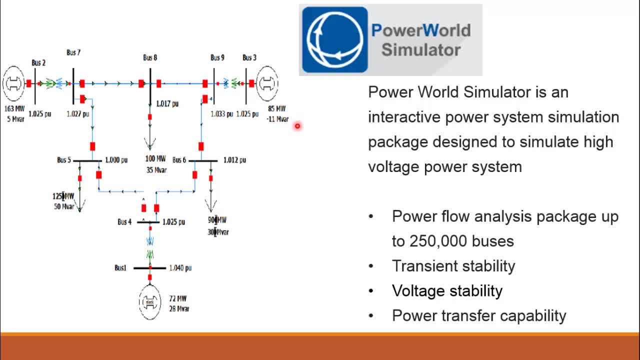 most powerful software for the electrical power engineers, in which you can have the ability to simulate high voltage power systems. You can also perform power flow analysis for up to 250,000 buses Once you have drawn a power system network. you can also perform the transient stability. 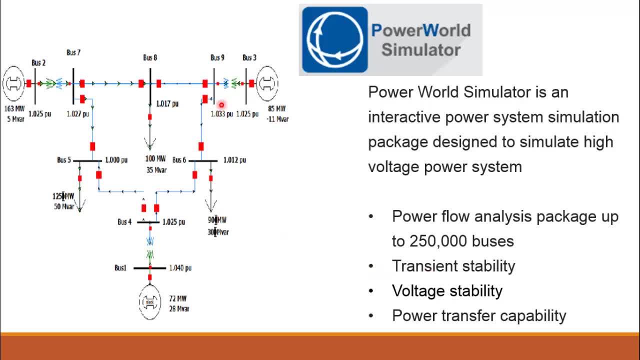 analysis and the voltage stability analysis, and also you can perform the power transfer capability of different solar systems. Next on our list is the PSPICE or the ORCAD WP-SPICE. This is a circuit simulation software. You can perform this very simple operation in the power system network. 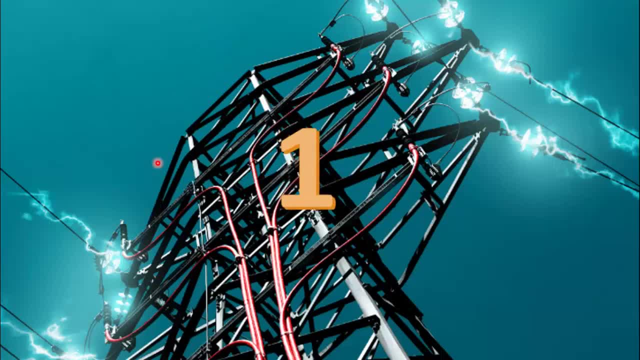 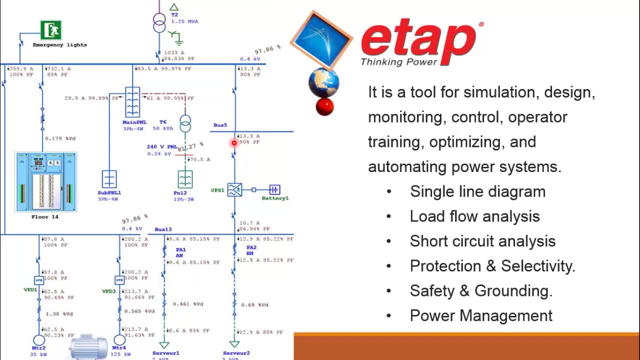 The last but not the least on our list is the ETAP. The ETAP is the most preferable software by any electrical design engineer. It is a tool for simulation, design, monitoring, control, operator training, optimizing and automating power system.